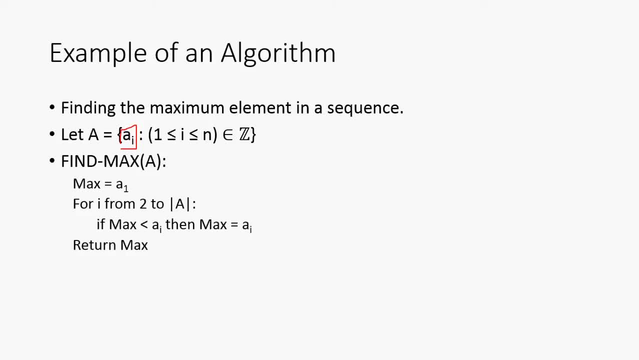 So I'm just going to define this algorithm to find max. so it's going to first set the max equal to the first element and then for i from 1 to the size of a. we just loop through it, essentially because there's four loops. So for each time we add a new element, it's going to loop through it. So, for each time we add a new element, it's going to loop through it. So for each time we add a new element, it's going to loop through it. 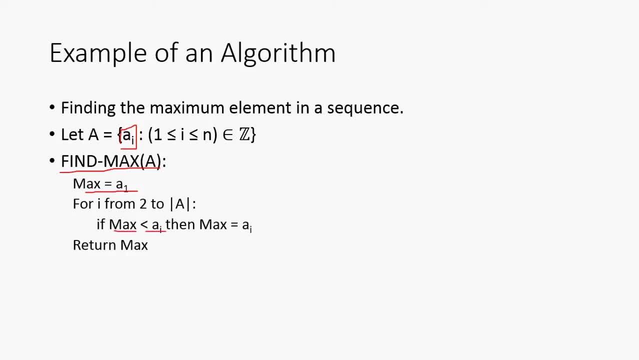 And if we look at each element, we're going to check if the current mass is less than the current element, And if it is, then we set mass equal to the element. And let's say, we go through the whole thing and we don't seem to do things well. that means the first element is a max. 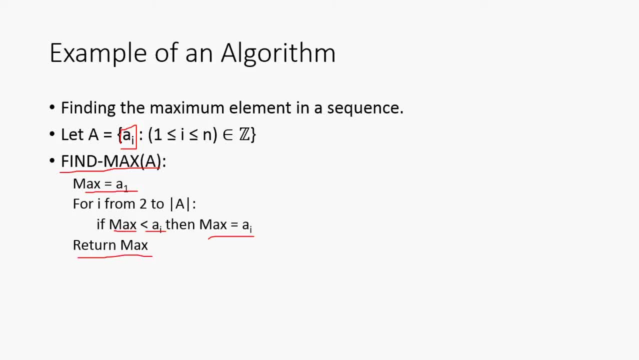 And we don't seem to do things well. that means the first element is a max, So we retain it. Otherwise it'll be some other element, And that's when you find the maximum element in, like a list or something. 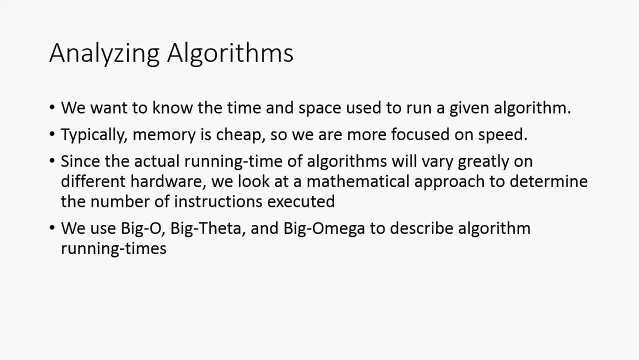 So typically we want to know the time and space used to run a given algorithm running given algorithms. So since memory- relative to time anyway- is steep, we're more focused on speed. So since the actual running time of algorithms will vary greatly on different hardware, 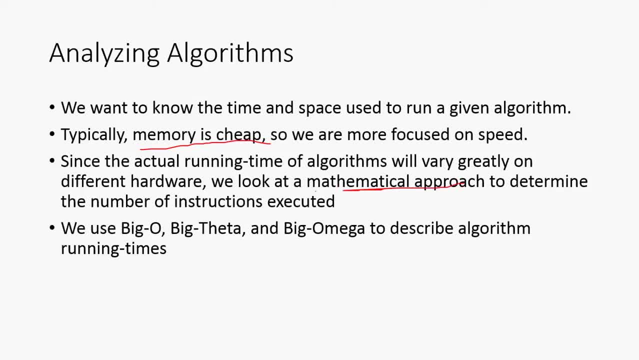 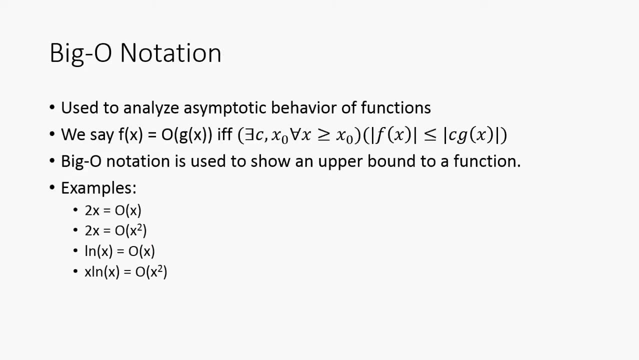 we look at a more mathematical approach right to determine the number of instructions used, And to do this we use big O, big theta and big omega to describe the running times of algorithms. So big O notation is going to look something like this: We use this to analyze the asymptotic. 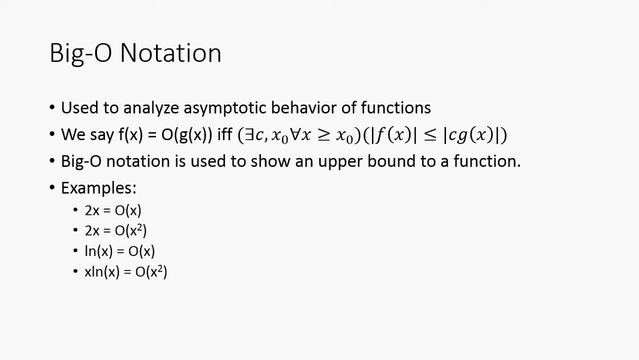 behavior of a function. This is going to be sort of the upper bound, I guess you could say, of a function. So we see that f of x in function is big O z of x If, and only if, there is this constant c and x naught for all, x greater than x naught, such that the absolute value of f of x 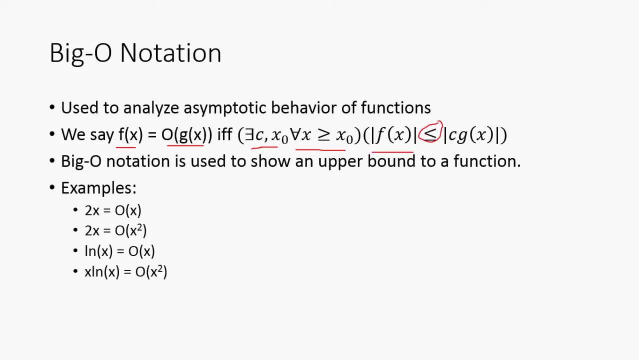 is less than or equal to the absolute value of some constant times g of x. So it's used to show sort of an upper bound to a function. So applying this sort of definition it looks kind of abstract. but if we sort of apply this definition as an example, 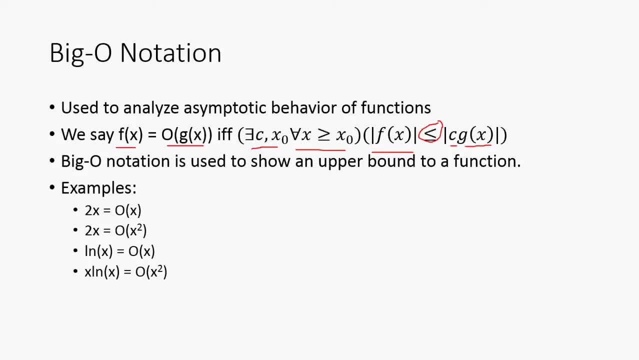 this might become a little more clear. So, for example, 2x is going to be big O x, right, because that just differs by a constant and that will work for any x naught, right. And 2: x is also big O of x squared. So if we take some x squared, if we take some x naught, 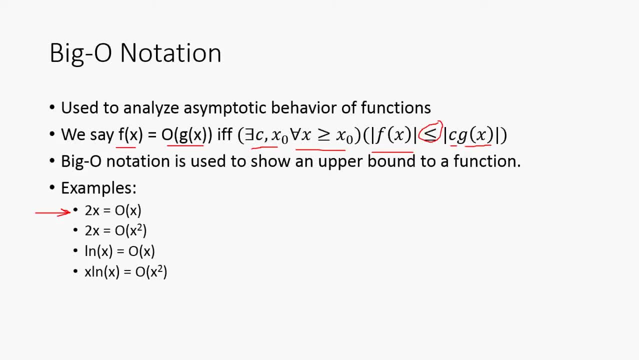 let's say 2,. clearly this is going to be. this relationship with less than or equal to is going to hold for x squared Right. and then let's see max. the log of x is going to be big O of x. That's because, if you look at the graph, 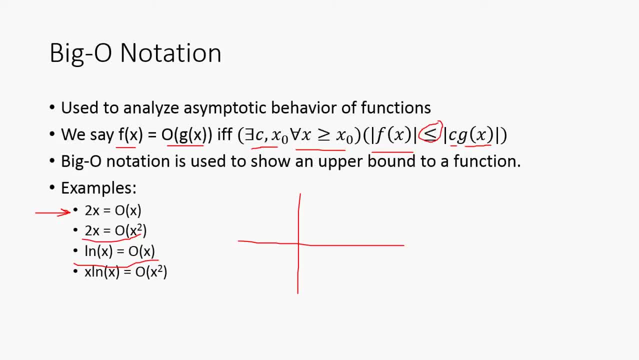 it's going to be a big single factor, And then x- t is going to be something like this Very roughly, And then, as we define the Frederickian values, we'll see that x log x is going to be equal to a big O of x squared. just by combining these two relationships right here. 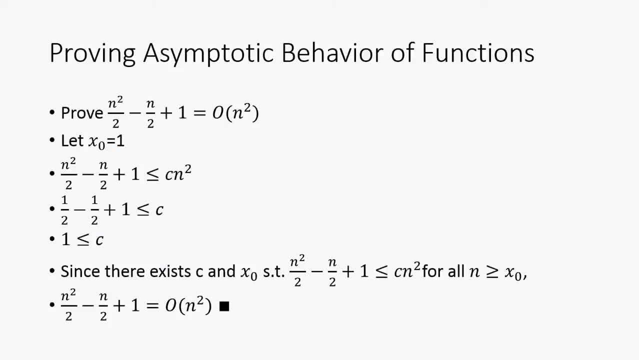 So now we can do some proof for the f-composite behavior function. So let's prove that this quadratic right here is a big O of n squared. So let's go ahead and prove that. First we'll choose some x naught right. 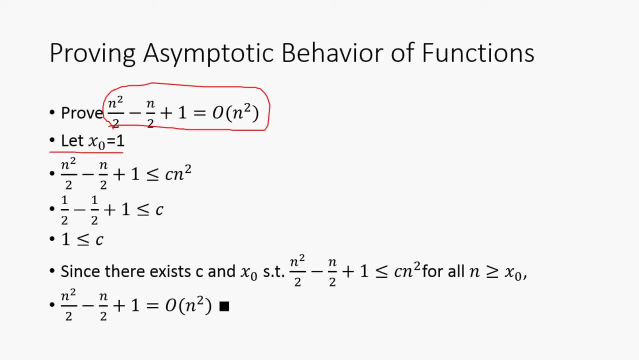 We'll let x naught be 1.. And then we're going to find a constant based off of this x naught to see if this relationship will hold. So this is our function, that we're comparing right here, And we're going to plug in our x naught and we're going to get that 1 half minus 1 half plus 1 is less than or equal to c. 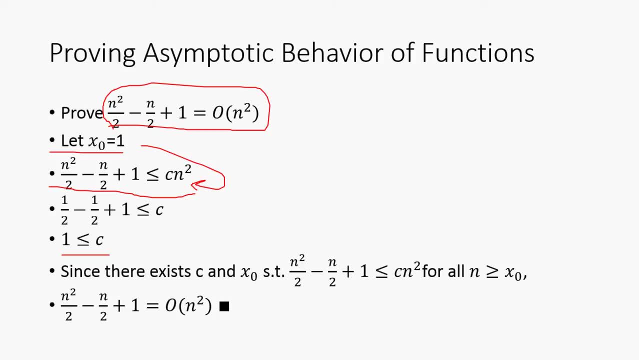 So we have to choose a c that is greater than or equal to 1.. And since we can find constants c and x naught such that this relationship holds true for all of the n greater than or equal to c, we're going to plug in our x naught. 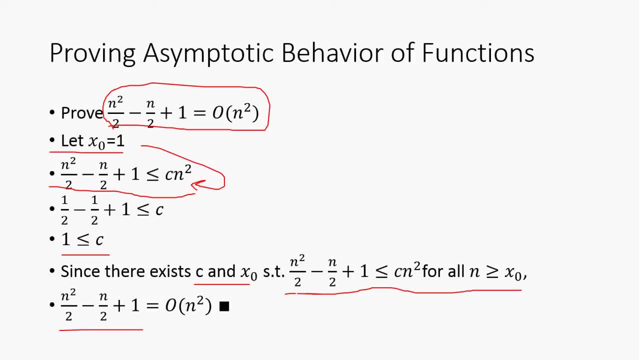 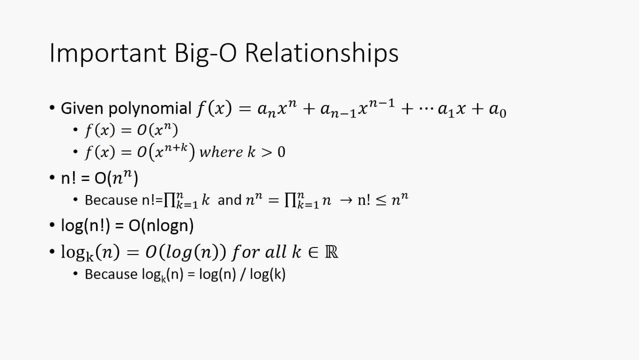 And this function right here: n squared over 2 minus n over 2 plus 1 is going to be big O of n squared. That's the way to prove. So this is an important big O relationship that you have to be aligned based on the terms of this. 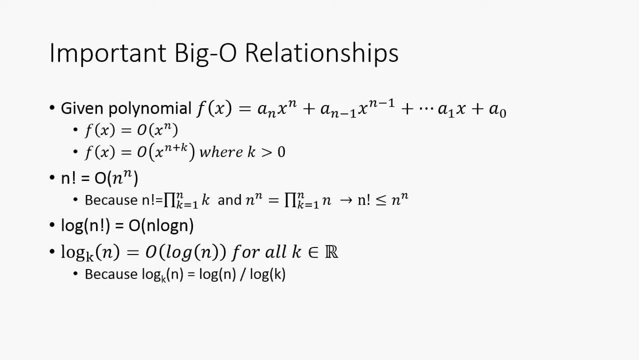 So if we get some polynomial, that's in the form of, like, some coefficient times x to the n plus some coefficient times x to the n minus 1, and then so on. So if we get some polynomial, this function right here. this polynomial is going to be big O of the degree of the polynomial right. 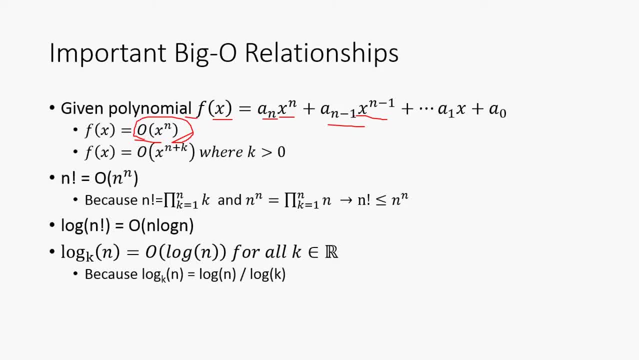 So it's going to be big O x to the degree. So, right here, it's big O x to the n, because the reading coefficient, sorry, sorry, the degree of the polynomial is n, And it's also important to keep in mind that it can also be larger than the degree. 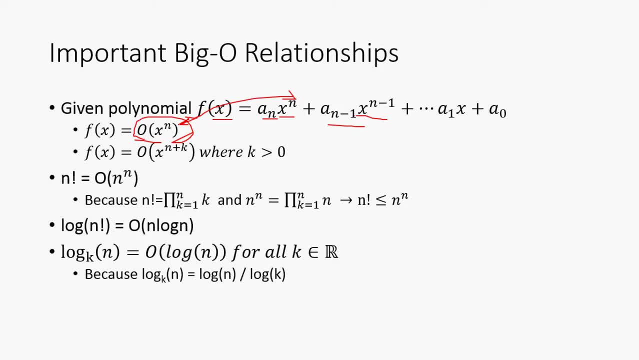 So that's true, It can be bigger than or equal to the degree for the big O anyway. So it can be x to the n plus k, where k is some positive number. So x squared is going to be big O. just to give you an example here: big O of x to the 2.5, right. 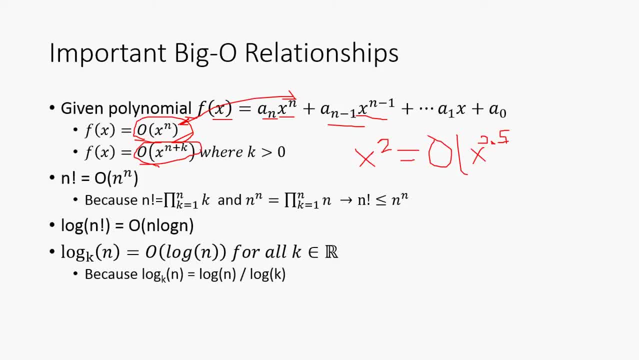 Because clearly it's big O of itself, x squared. but it's also going to be big O, It's also going to be bounded from above by a function greater than x. And then another important relationship is going to be n factorial, which is big O of n to the n. 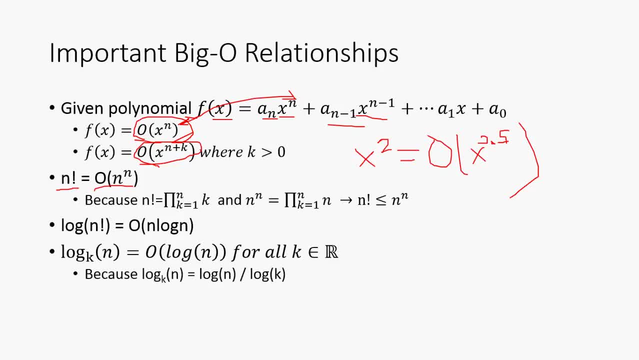 And we'll use this fact later on because it's pretty useful. We see n factorial a lot in common course And if we try to run an algorithm over a common factorial problem, this is going to come up. So, because n factorial is going to be a product of n terms and it's going to be, you know, one, two, three, four, all the way up, right? 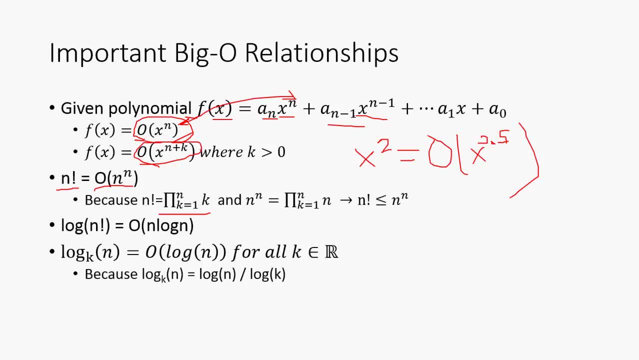 And n to the n is going to be a product of n terms, but they're all going to be n, so it's going to be upper bound. It follows that n factorial has to be less than or equal to n to the n right. 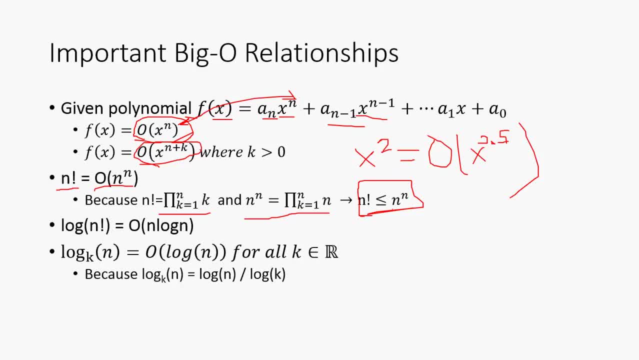 There's just no way you can get around that. So this is an important relationship, but not as important as this one right here where we apply the logarithm. So the logarithm is factorial, which you might see- Oh I don't know- in like MergeSword or something. 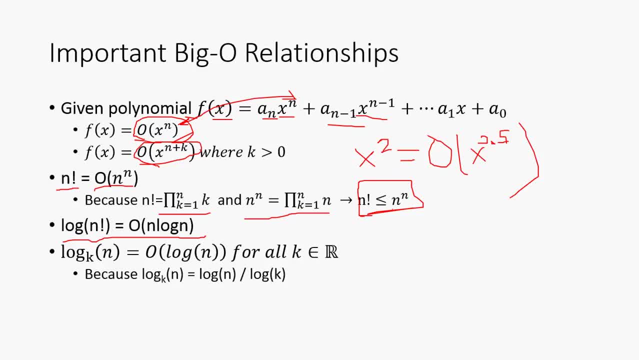 It's going to be big O of n log n, right, And that happens to be the running time of a bunch of shorter functions like MergeSword and QuickSword. So big O n log n because of the power rule, logarithm right. 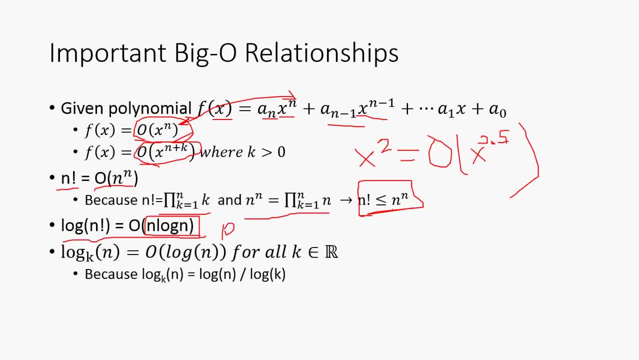 So if we have log, I can't write it log of a to the b right It's going to be b log, okay, because the exponent is getting moved out from the log. And then another important property of logarithm that'll be important for big O notation. 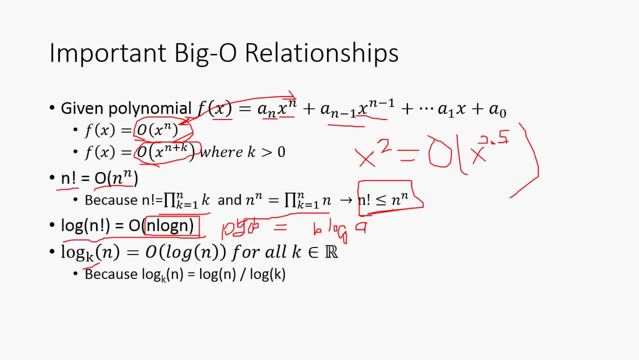 is that the log base, something of n? it doesn't matter what that something is, is just going to be big O of log n, right? Because log base k or log base k, for whatever it is, is going to be the log of n over the log of k. 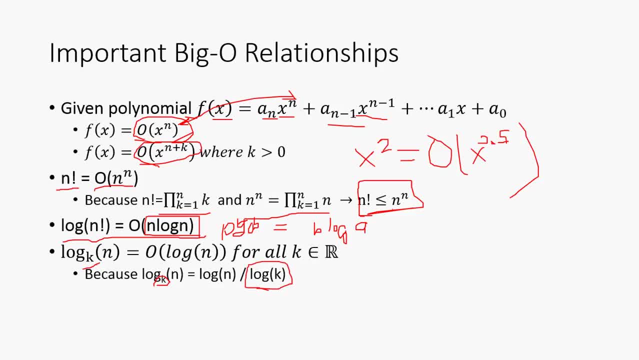 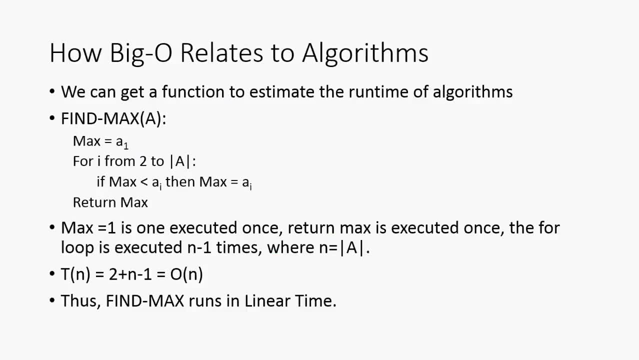 And the log of k is going to be some constant right, So it doesn't affect the asymptotic behavior of the function. So how big O is the algorithm? Well, we can find a function that estimates the running time of an algorithm. 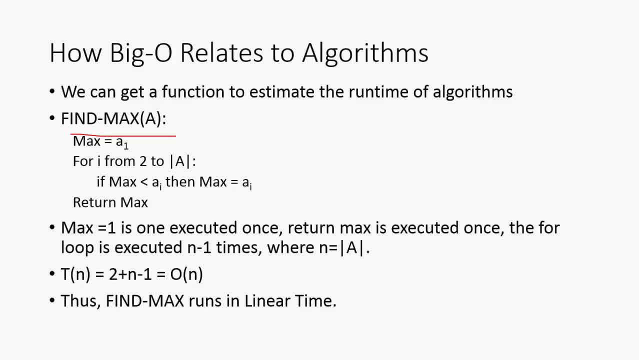 So consider our example to find that right. This right here. right here, this mass equals a1, that just takes one instruction. right. And this right here, this return mass, that only takes one instruction as well, right, So it's only run once. 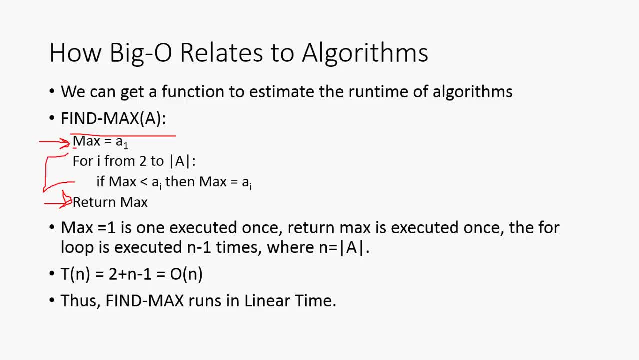 However, this for loop right here, this for loop runs from 2 to the length of a. So if we just let the length of a equal n, this is going to run n minus 1 times right? So if we write a function called p of n that models the running time of this algorithm, 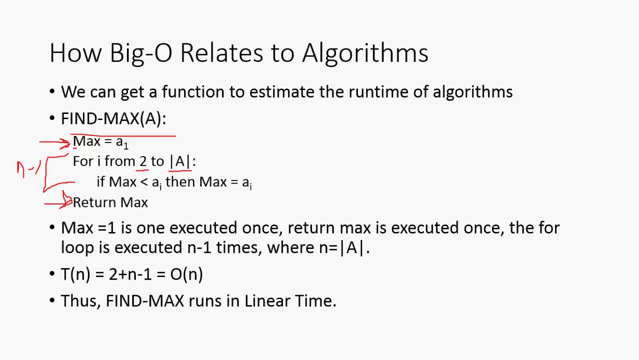 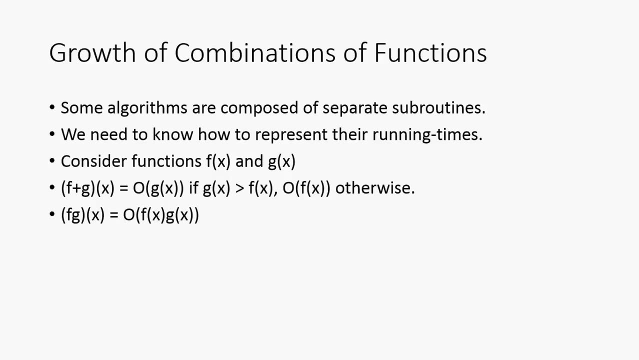 it's going to turn out to be: p of n is equal to 2 plus n minus 1, right, And that is big O of n, based off the properties from the last slide. So because of this, because it runs in big O of n, we say that firing mass runs in linear time. 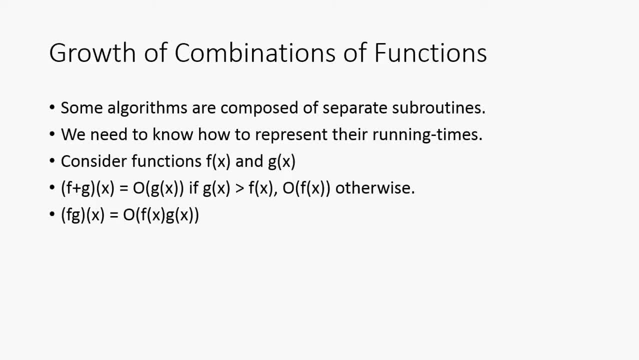 So next we'll talk about the growth of combinations of functions. So some algorithms are composed of separate separations or functions within functions, right? So we need to know how to represent them. We need to know how to represent these different combinations or compositions, right? 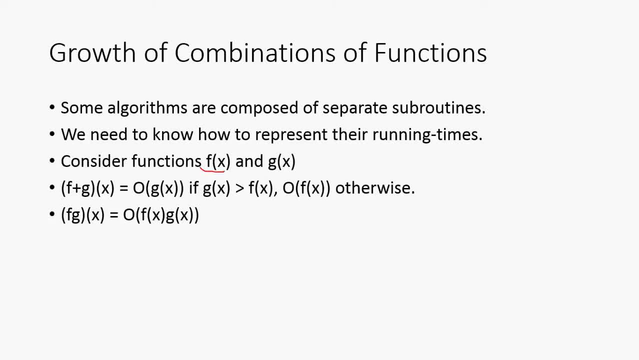 So let's consider two arbitrary functions: f of x and g of x. So if we add two functions together, as represented by this composition notation here, then it's going to simply be g of x, if g of x is greater than f of x. 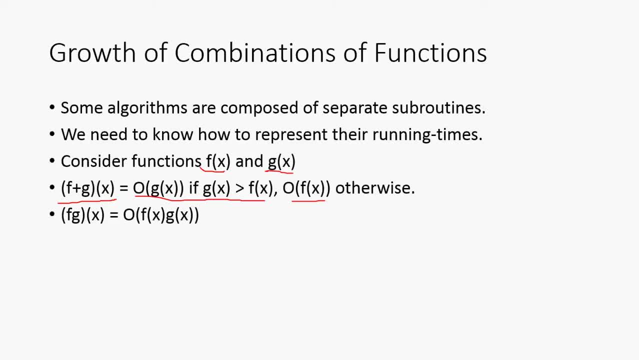 or it's going to be f of x otherwise, So it's just going to be the bigger of the two terms, essentially, Right? So, and then for the product, for the two functions, right here, f of g of x, it's simply going to be the big O of the product, right? 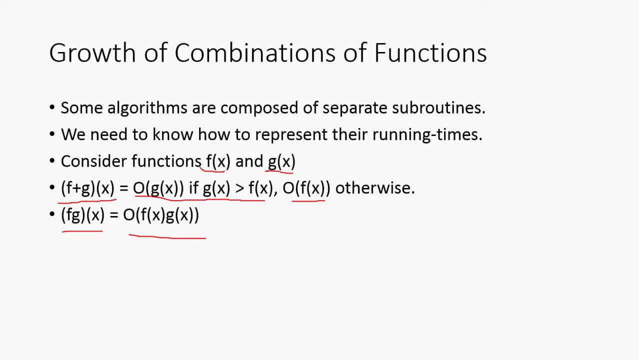 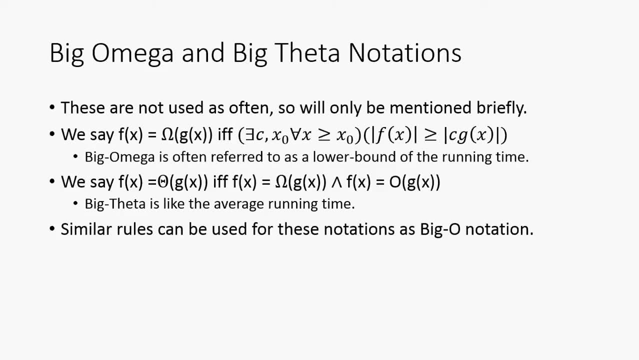 The product of the big O. So we discussed big O for a while. Here's the upper bound. Next we're going to discuss big omega and big theta. Now these aren't used as often, so I'll only mention them briefly, But I'm going to provide the formal definitions right here for big omega. 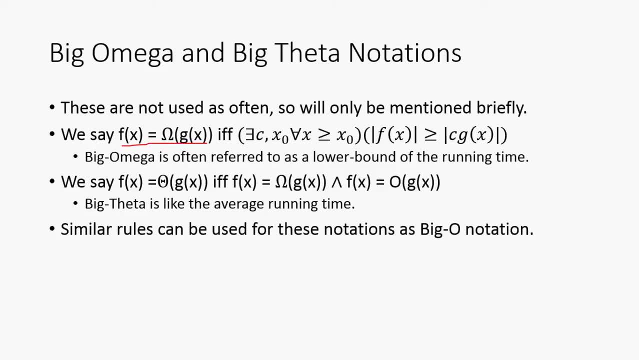 So we'll say that f of x is big omega g of x if, and only if, right, There exists two constants, g and x naught. for all, x greater than x naught, such that the absolute value of f of x is greater than or equal to 2, right. 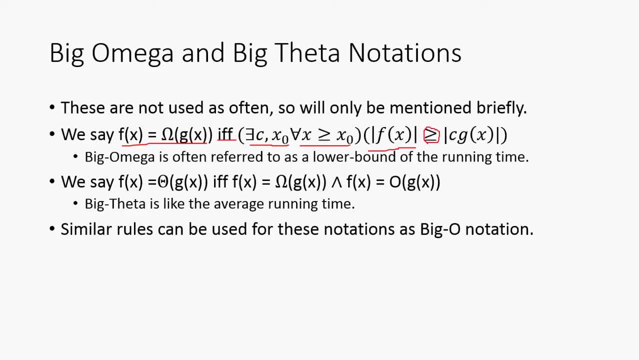 And so this is the opposite of the sign for big omega. you see, right, Because big O is kind of an upper bound, right? Well, big omega is going to be a lower bound, So that's why we put the sign here. 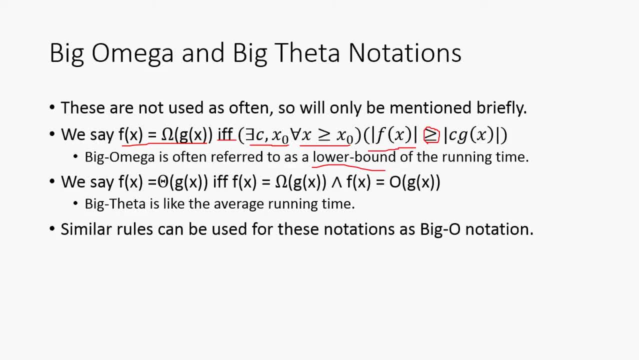 So it's going to be better or equal to the magnitude of c times g, of x right, And c is the function. So this will just give us the running time, the lower bound of the running time, right, And finally we have big theta notation. 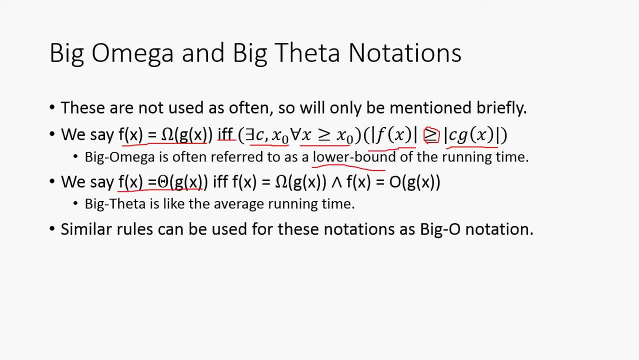 So we say that f of x is big theta of g of x if, and only if, f of x is omega of g of x and f of x is big O of g of x. So big theta is like the average running time.